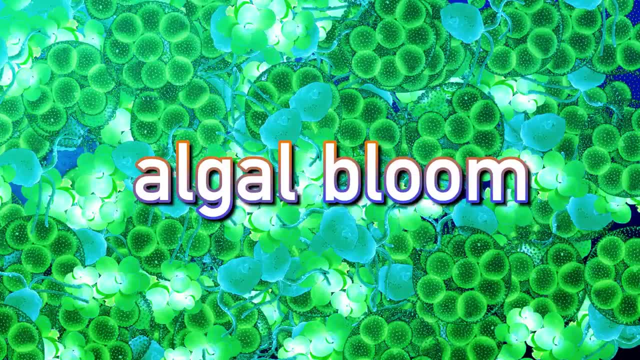 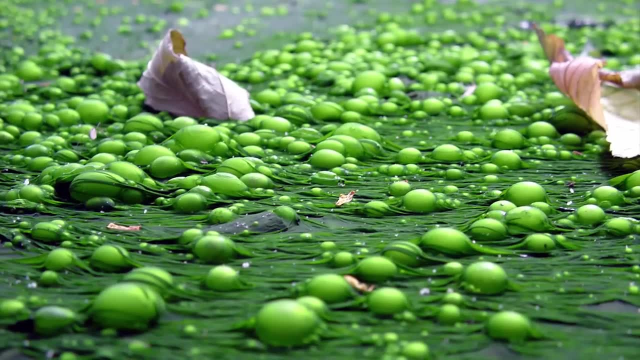 and entire lakes can become covered in layers of plant growth like this. To some, this might seem like a weird thing. Plants are good for the environment, right? Well, not always. First off, this floating layer of algae forms basically an impenetrable roof on the water, not allowing 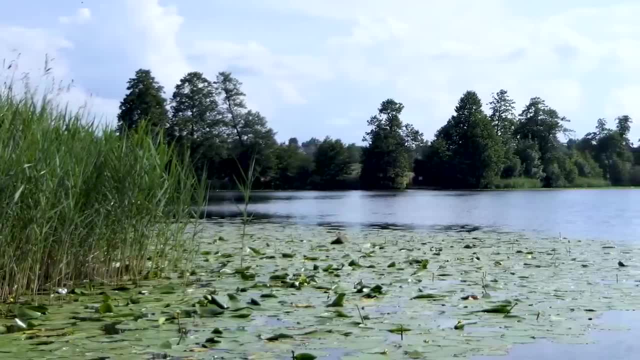 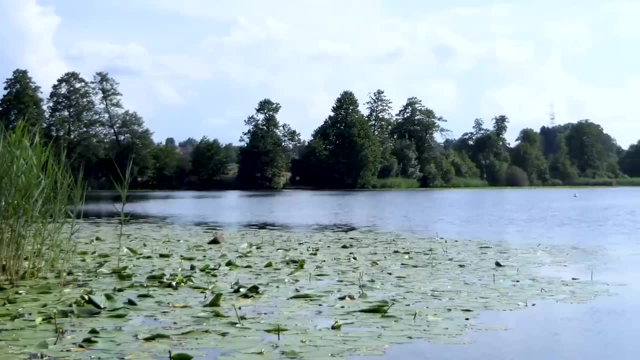 sunlight through to the bottom of the lake. Without the presence of sunlight, all plants below the surface cannot partake in photosynthesis, You know, metabolize, make glucose, live that sort of stuff. But not even this is the bad part of it all. Many plants can store enough. 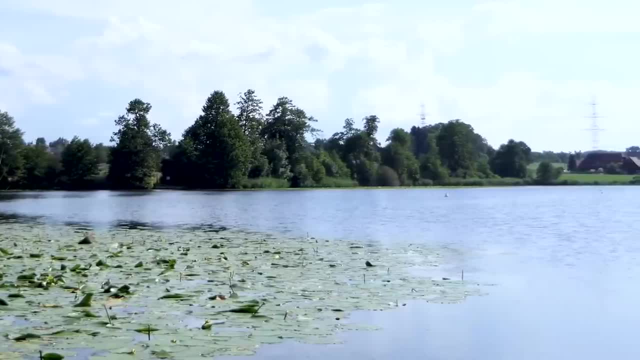 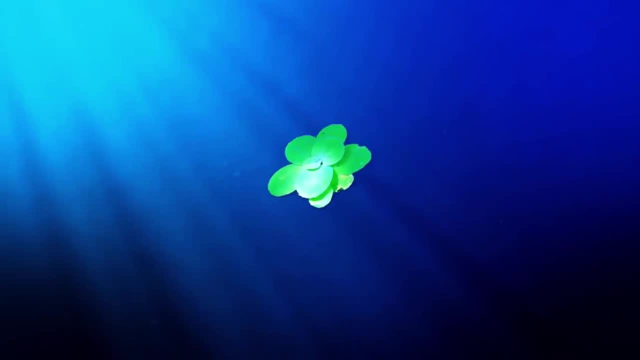 energy in their bodies to wait out these conditions. The real problem comes when all the nutrients are used up and the water can no longer survive. When this happens, the excess algae, phytoplankton and plants die off and sink to the bottom of the 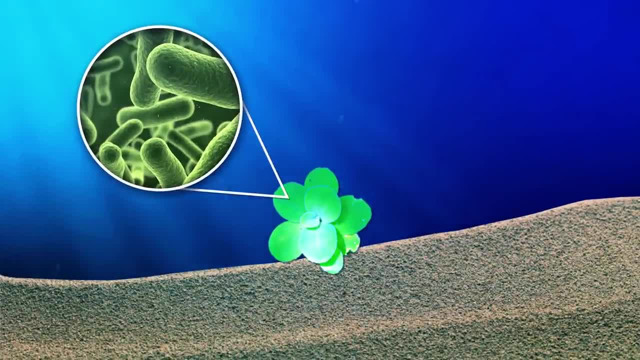 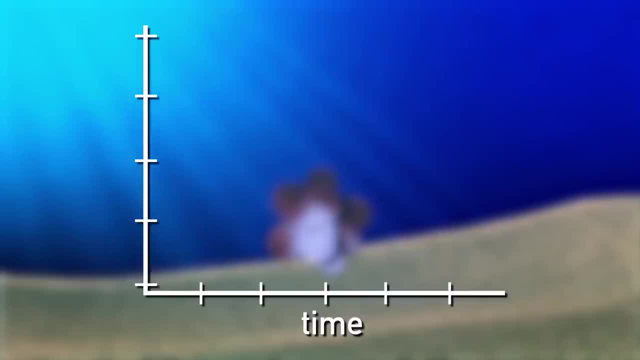 body of water. Here bacteria and other decomposers feast on the dead bodies in a chemical process of decay which consumes oxygen. Now, in a usual ecosystem the amount of dead matter is relatively constant, so oxygen levels stay relatively constant as well. But when a bloom occurs, far 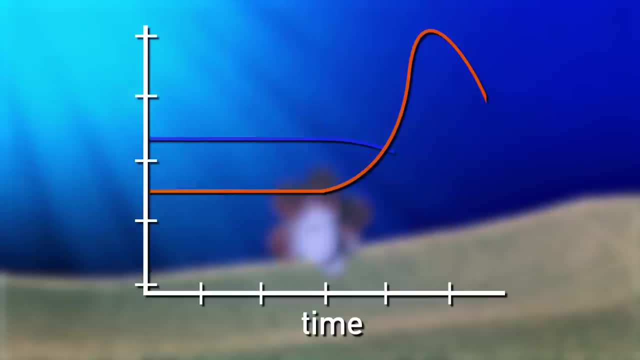 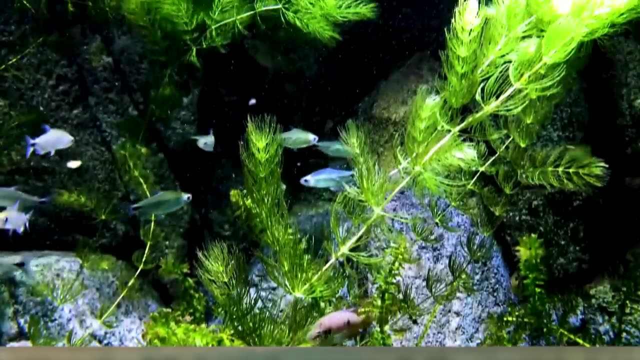 more organic matter is ready to decompose, and so nearly all the oxygen in the water is used in the body of water. This causes even more death, leading to more decomposition, and none is left for the animals living in the water Without this, animals that use the dissolved oxygen to breathe. 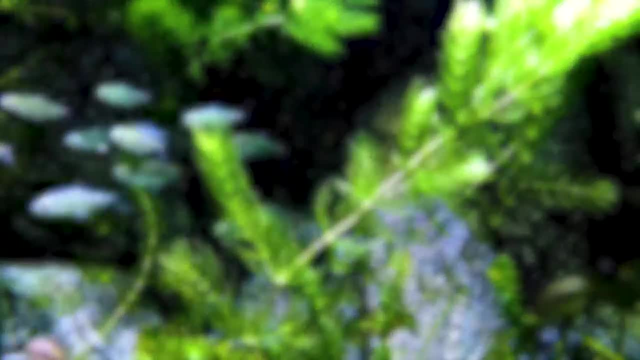 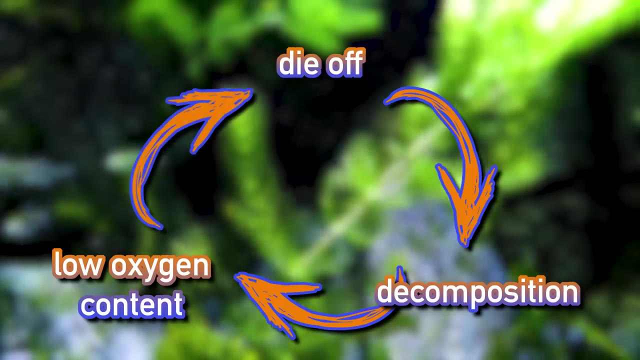 so things like fish can actually suffocate. This causes even more death, leading to more decomposition and more oxygen usage. Basically, at this point, a positive feedback loop has been created. It can take a body of water a very long time to recover, though each one is different. 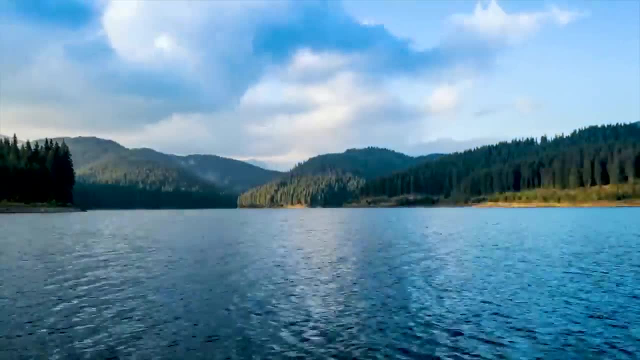 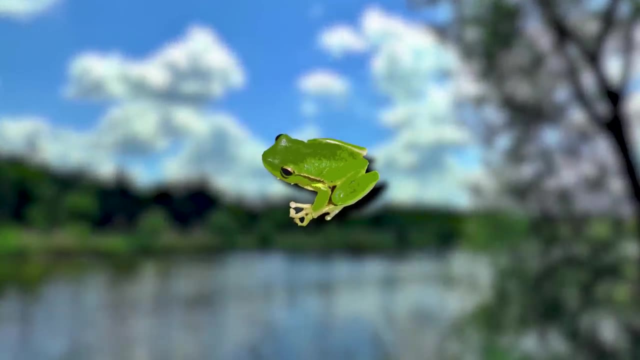 and recovery depends on a lot of things like how many nutrients leaked into the water, how big the body of water is, what organisms are present there, and so on. When this happens in the ocean, native species can be suppressed and allow invasives to come in, while the environment 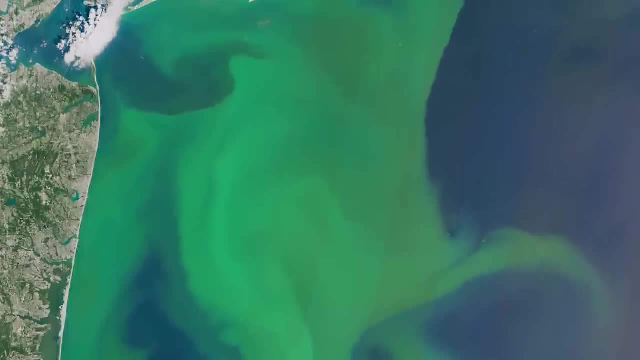 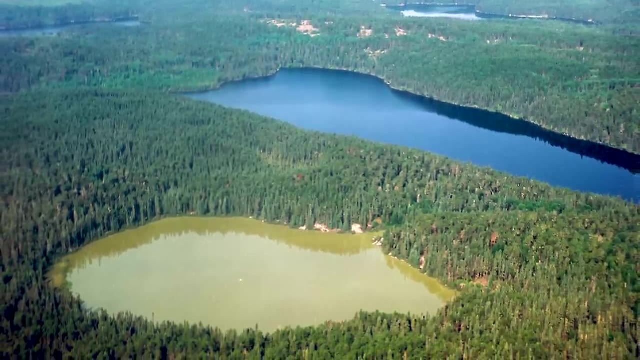 is still disturbed. If this happens in the ocean, the lack of oxygen can cause corals to bleach and possibly even die All around. this can greatly damage many ecosystems and leads to a decrease in biodiversity globally. Nutrient-rich runoff can also be caused by things like clearcutting. 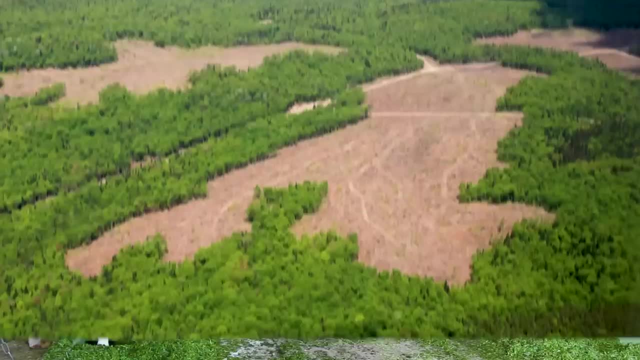 which releases the nutrients which were kept in the soil by the plants or also by things like animal farms, where nutrient-rich waste materials can leak into local bodies of water, And that's eutrophication, simply because of the amount of water in the water and the amount of water in